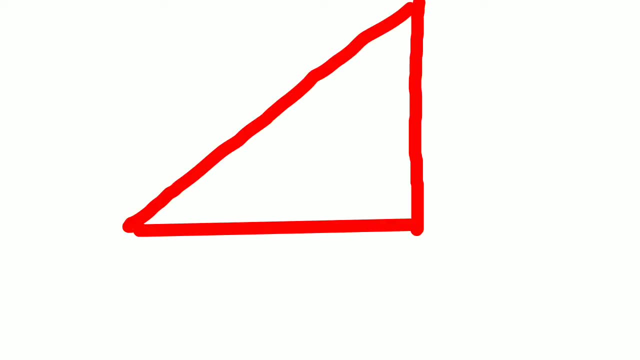 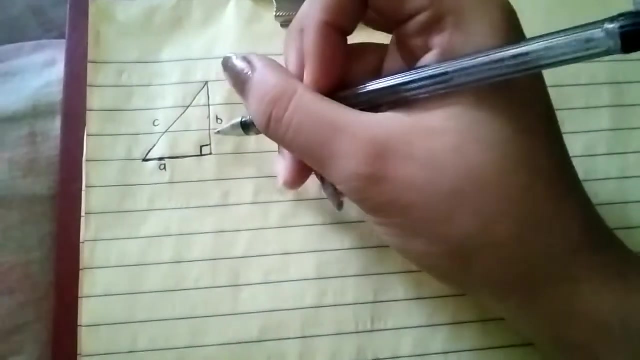 In Pythagorean theorem, triangle should be right angle. Longest side of triangle is opposite to the 90 degree angle and it is called the hypotenuse. These two adjacent sides are called the legs of the triangle. A and B represents the length of the legs of the right triangle. 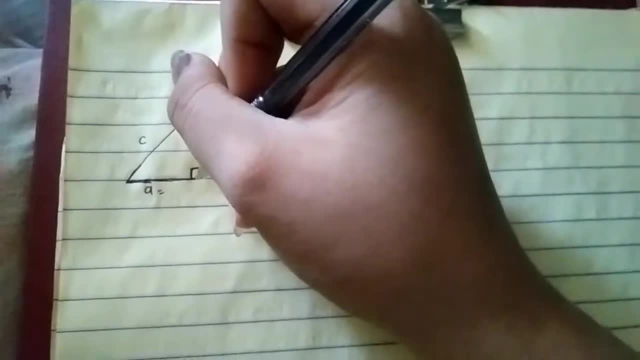 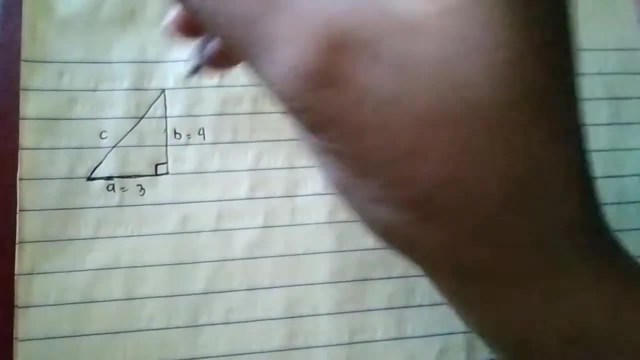 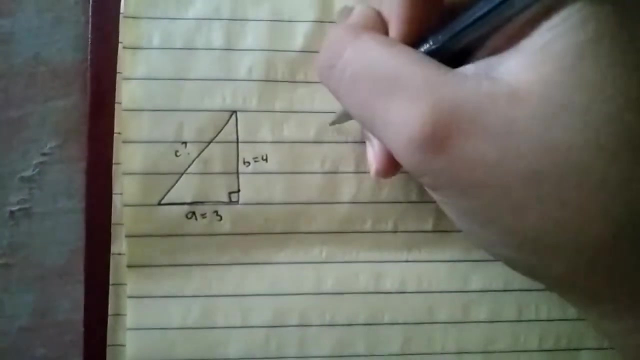 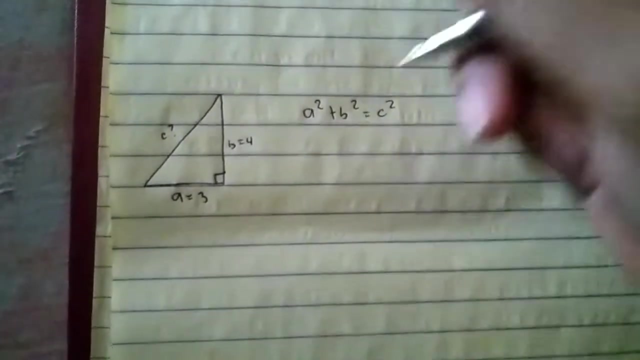 and C represents the length of hypotenuse, And then substitute 3 for A and then 4 for B, While C is the unknown. First we have to write the formula, which is: A squared plus B squared equals to C squared, And then A squared is equivalent to 3.. 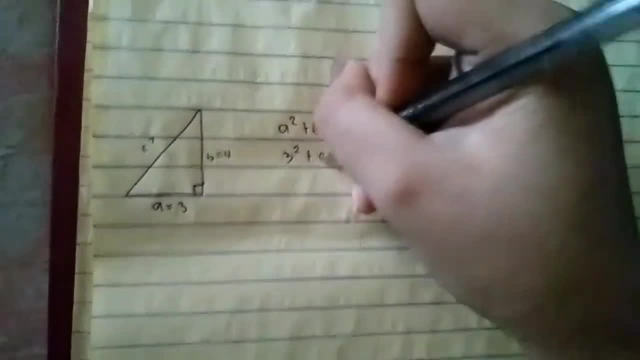 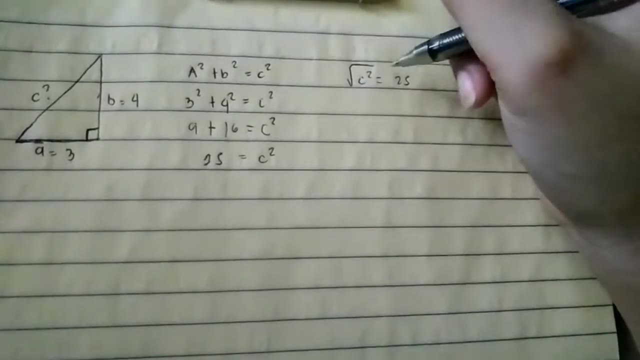 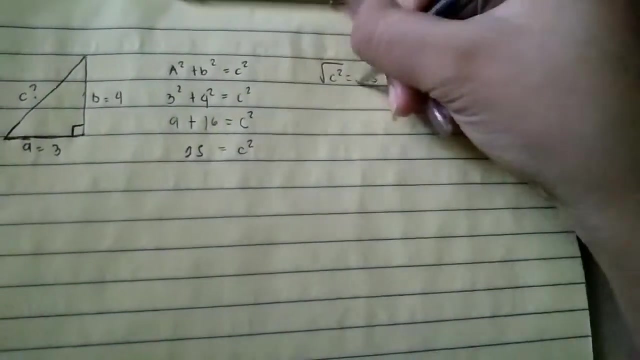 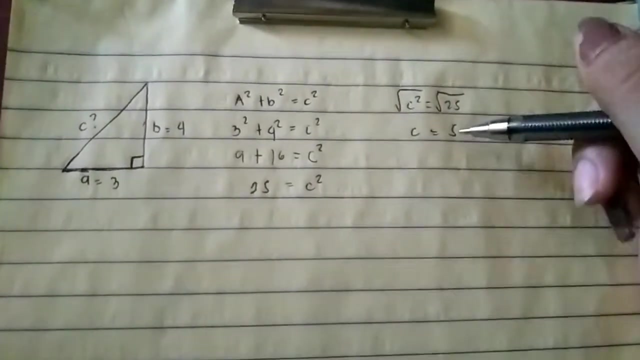 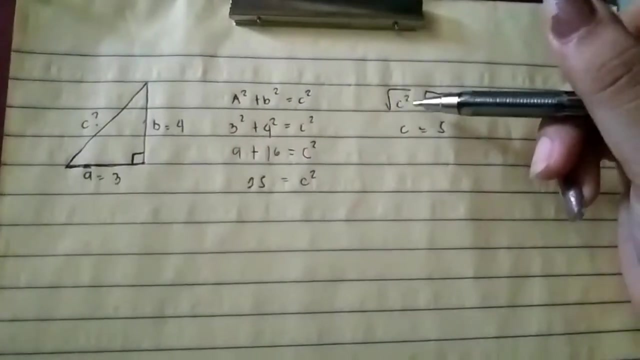 And B squared is equivalent to 4.. And then copy C squared And then copy the C squared equals 25 and put the square root both sides. Simplify the square root of 25 and the answer is 5.. Taking the square root of C squared, just give us a C, which is what we want on this side of the equation. 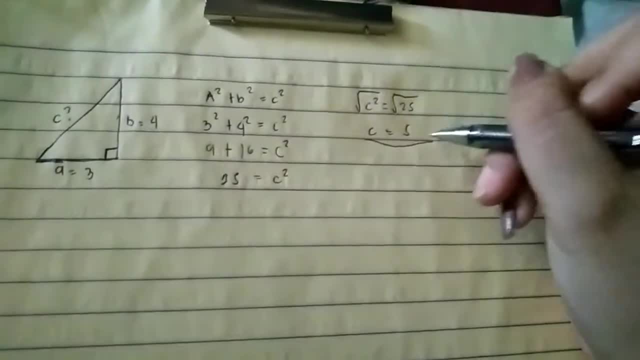 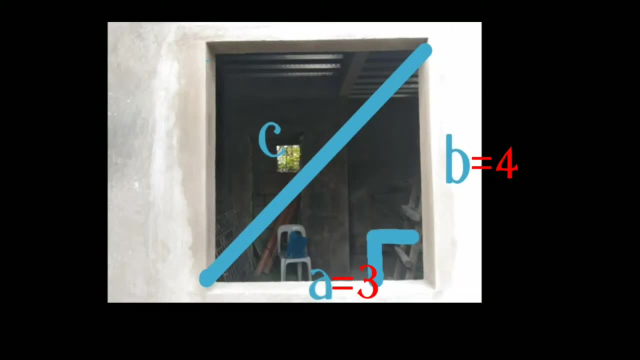 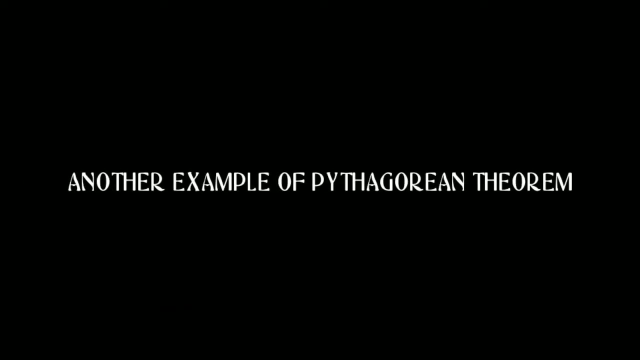 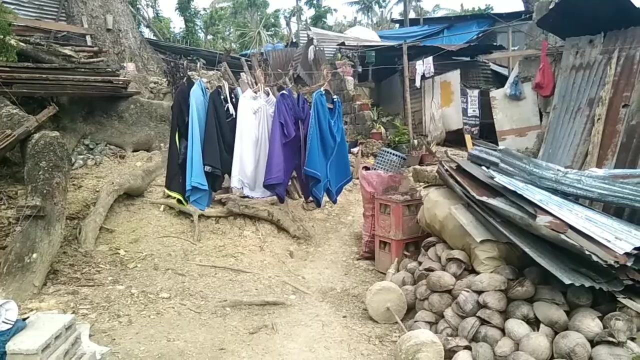 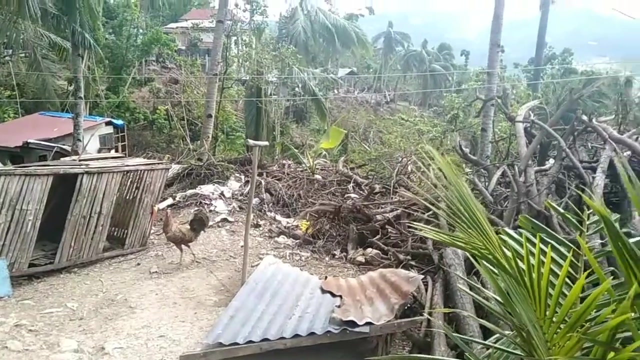 So the measure of C is 5. And that's the answer. So the diagonal of window is 5.. When I went home from my neighbor's house, I feel so hot like hell. Then suddenly I saw a fighting cock nearby which has no shelter to hide, or even the shade of a tree. 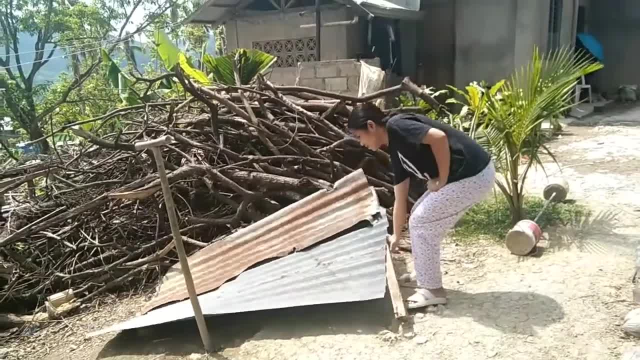 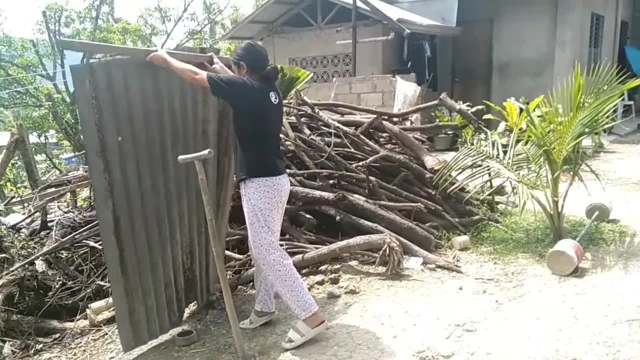 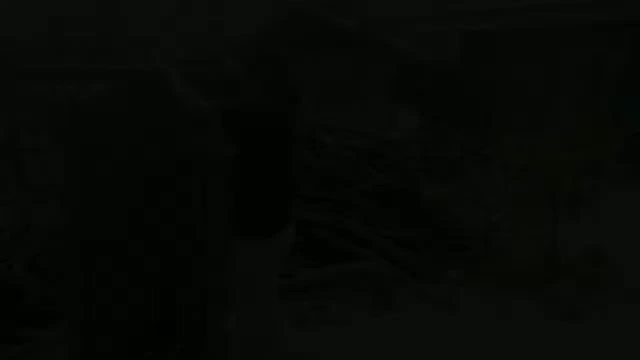 I walked through the fighting cock and what I did was I get the pieces of roof and cover him. I stand some pieces of roof, but it is not in front of me. It is not enough space. So I use Pythagorean theorem to know the measurement of space: big space. 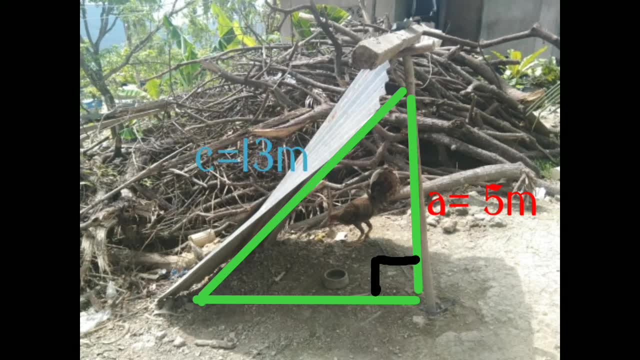 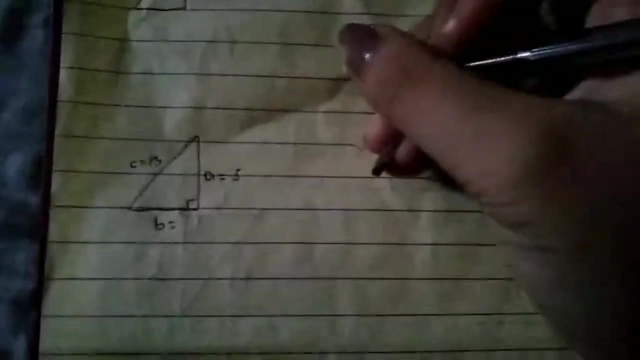 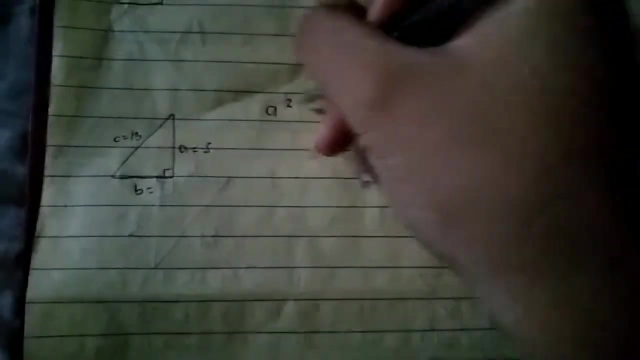 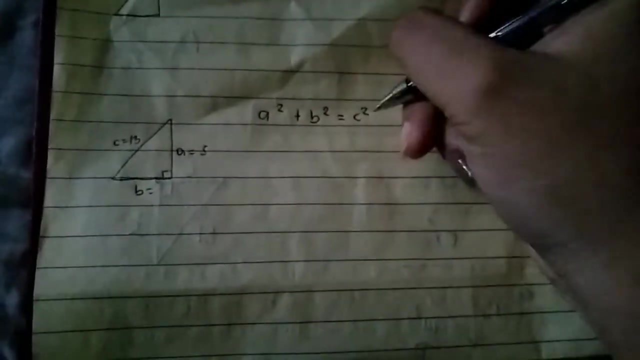 I measure the height and it is 5 meters long, and the size of a roof is 13 meters long. So to come up with the space, I need to solve the missing area. First we have to write the formula, which is: A squared plus B squared equals C squared. 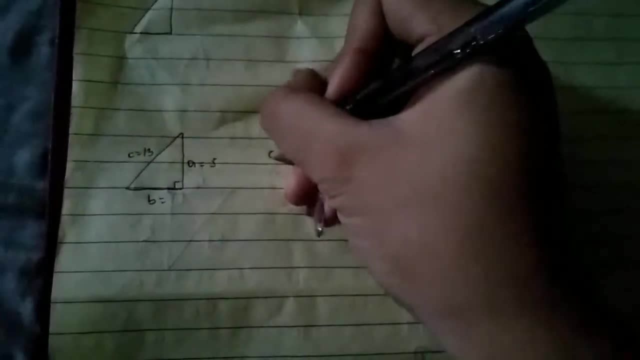 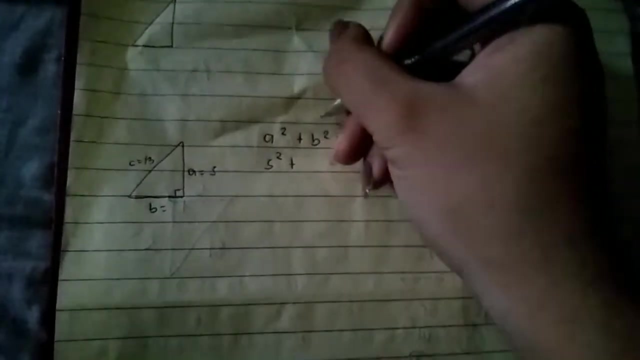 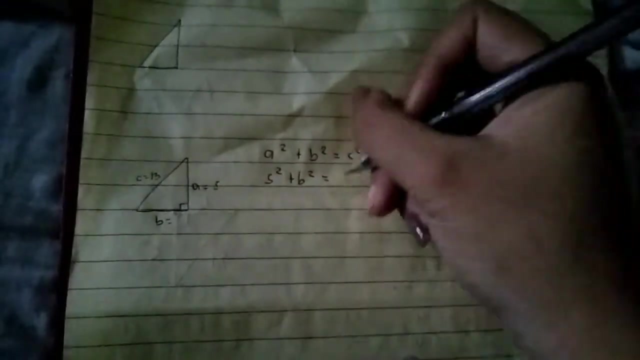 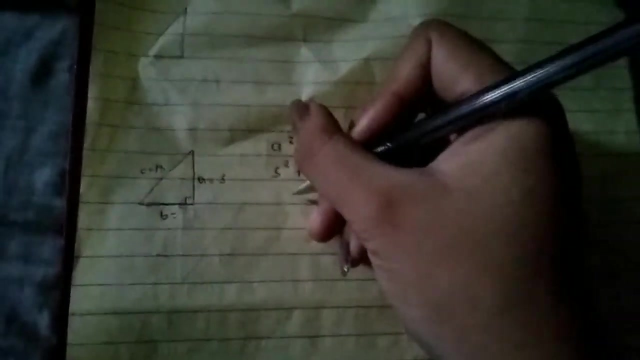 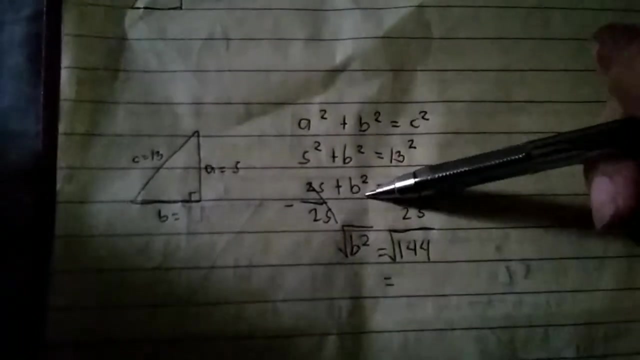 So A is 5.. And B is unknown. So copy the B. B squared equals The C squared is 13.. So 13 squared, Okay. so 5 times 5 is equals to 25.. Plus B squared is equals to 13 times 13.. 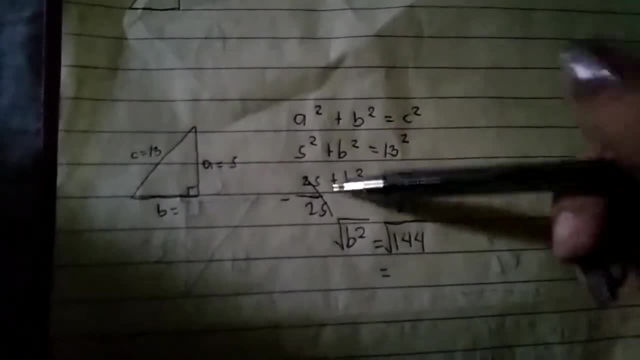 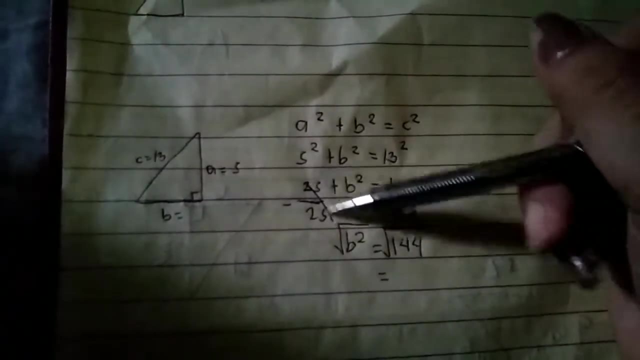 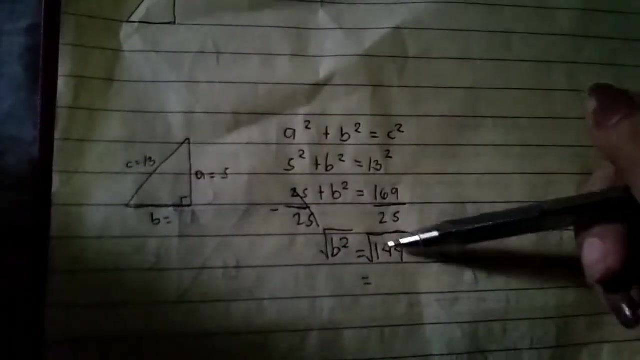 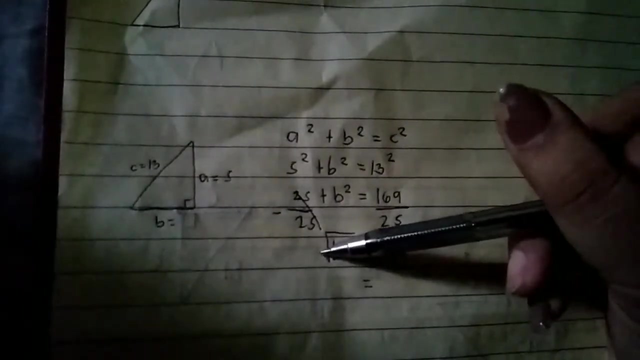 It equals to 169.. And subtract both sides into 25.. So brush out And 169 minus 25 is equals to 144.. And then bring down B squared And square root both sides And then simplify 144.. 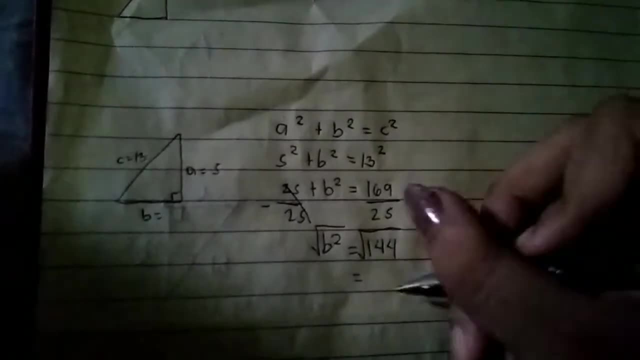 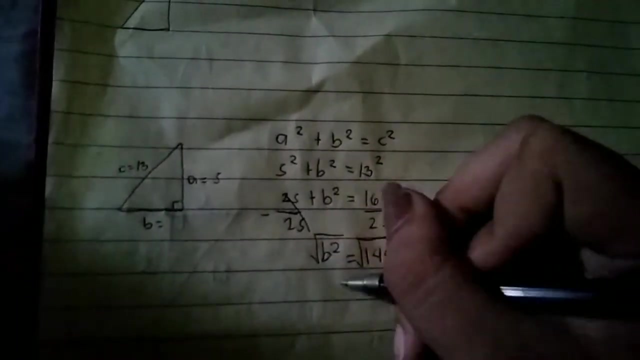 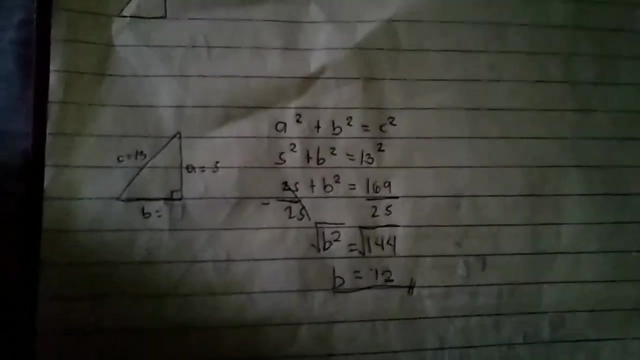 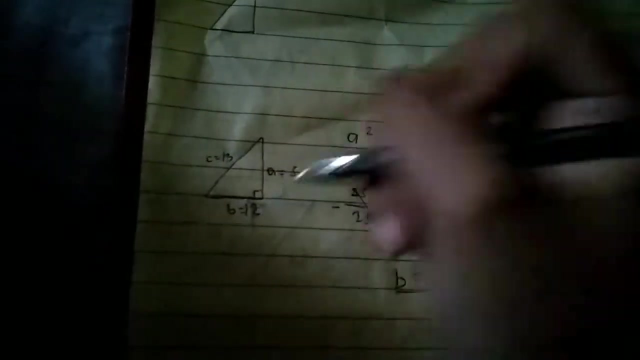 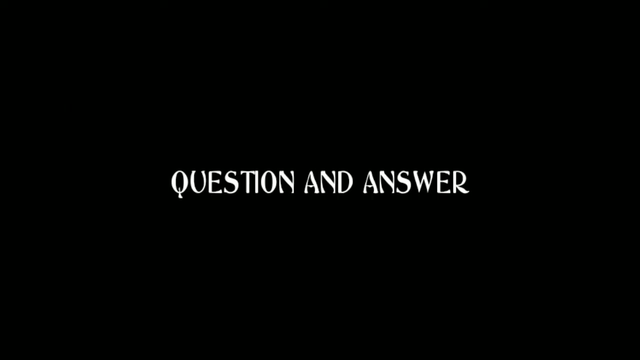 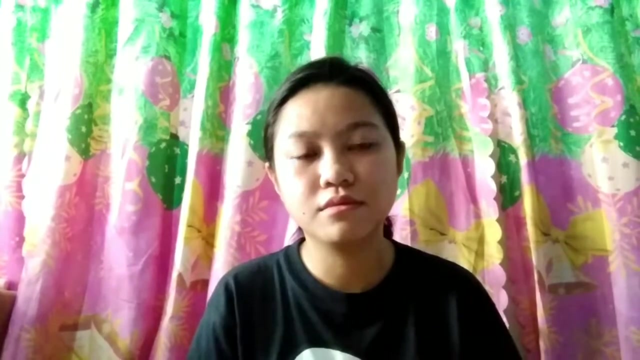 So the answer is 12.. 12. And copy the B, So our measurement of B is 12.. The measure of B is 12 meters. Do you think the Pythagorean theorem has been useful to humanity since Pythagoras learned about it? 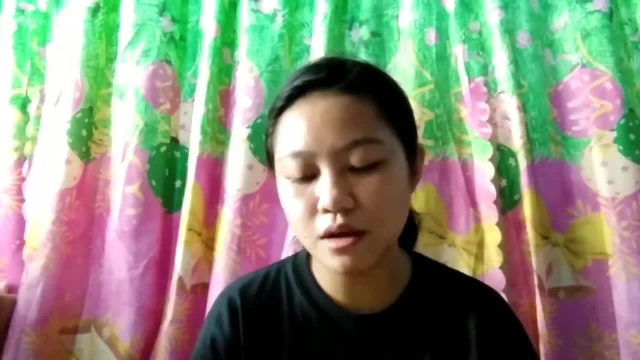 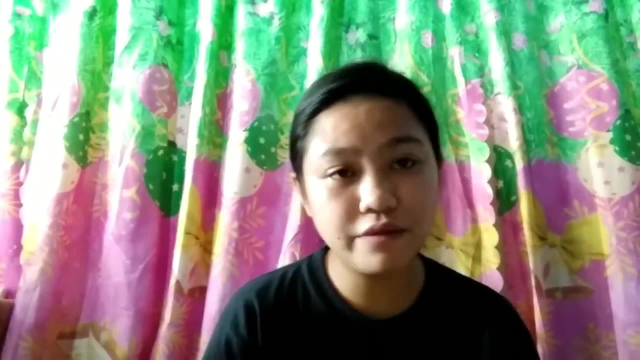 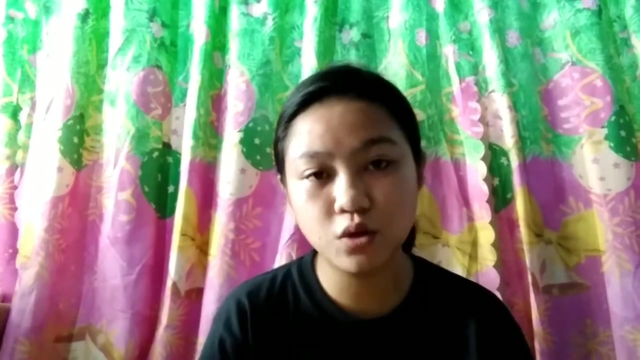 Explain your answer. Yes, Pythagorean theorem has been useful to humanity, Since it is used by the architectures, navigators, constructions and surveyors of the land, just like what we saw in a school building, houses, buildings or even skywalks.